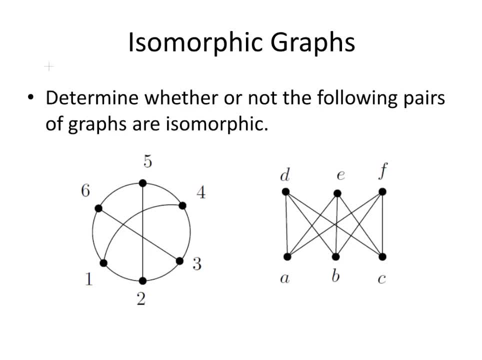 So we have- let's first off just check that they have the same degree: sequence: 3, 3,, 3,, 3, 3, and 3.. And likewise over here. it's pretty clear over here that they are both 3 regular graphs. 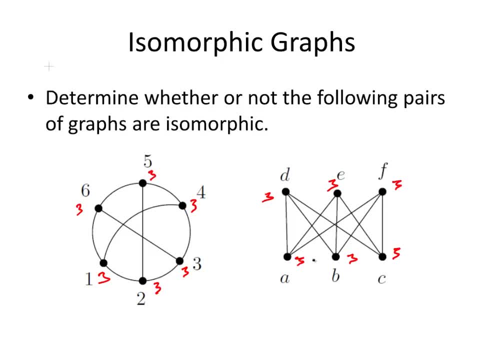 Okay, but is that enough? We're going to find out soon enough. Now, that's not enough to prove it. What we have to do is try and sort of look at the edges and just sort of see if there is an equivalence there. 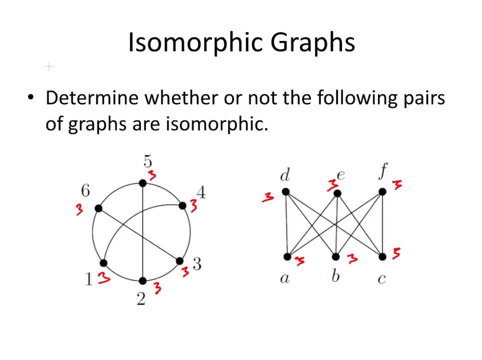 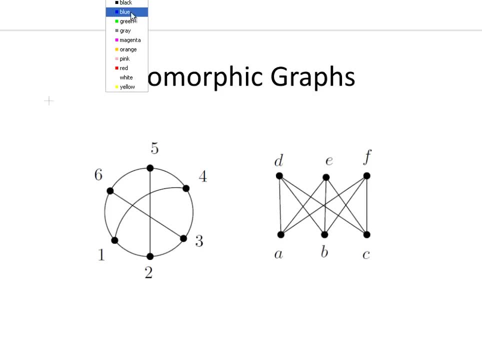 So what I'm going to do is I'm going to go to the next slide here now, And in the first instance, what I'm going to do is I'm going to see if I can equate Vertex 6 with vertex D. 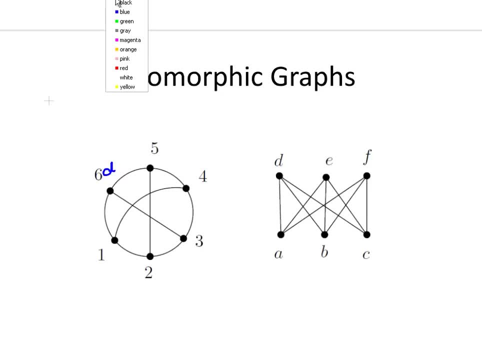 And what we're going to do is we are going to examine the edges of both sets of vertices. So, in the first instance, what I'm going to do is I'm going to- by the way, actually just as a remark- colouring in. bringing a sort of set of markers with you to an exam hall when you're doing. this is pretty handy. 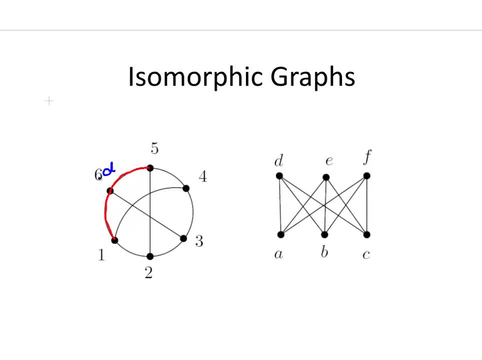 So what I'm going to do first off is the vertex from 6 to 5 and 6 to 1.. And I'm going to see if I can equate them to this one down here, A, And this one down here. 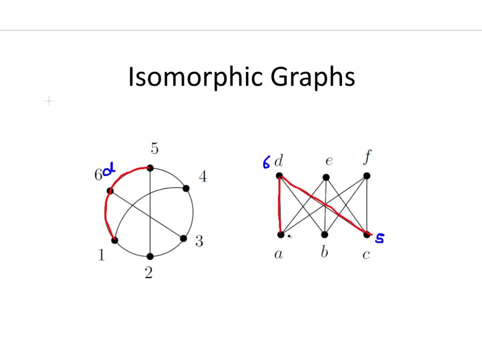 I'm going to let that equal 5.. I'm going to let that equal 1.. I'm going to let that equal C And I'm going to let that one equal A, Necessarily the one in between. It just actually uses as many colours as you can just to sort of make it as easy to follow. 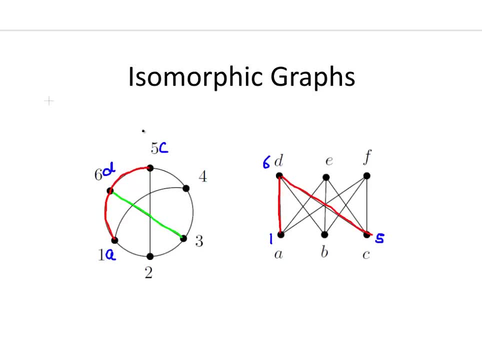 This one down here. I'm going to see if I can equate that to B. Okay, So let's do that same thing over here. Okay, Now The vertices that are connected to 1 and 5. Are, in other words, are in the other diagram, A and 6.. 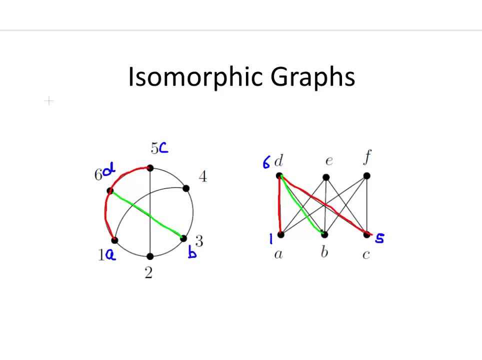 Are, in other words, are in the other diagram A and 6. Are, in other words, are in the other diagram A and 6.. they both connect to 4 and F. So let's do that, Let's go there. 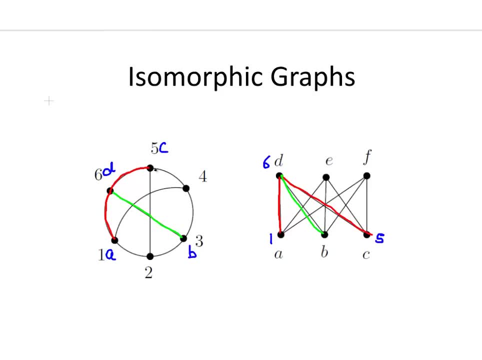 Let's paint them in orange. So this one here and this one here, And we're going to see if that equates to F, and this one here, And we're going to see if that equates to F Now. so let's do the same thing on the other diagram here. 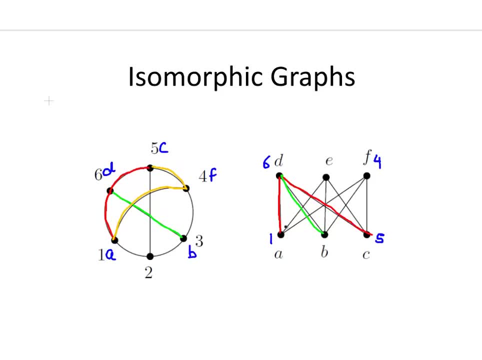 By the way, this is a very long approach now, So I'm not sort of pretending this is a quick approach, but it's just, it's a very you know if you are having any trouble with it, So I'm going to paint those ones up there. So that looks good so far. 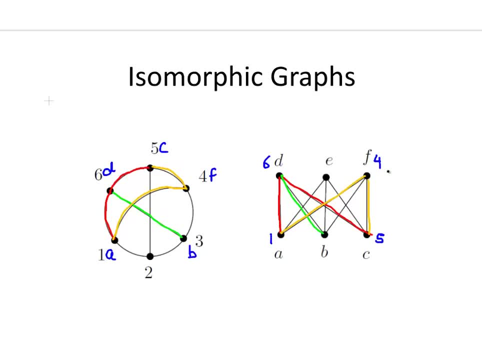 So now what has to happen is that B and A have to connect to C. So, essentially, what we're looking at is vertex 2, vertex B- Okay, sorry, by the way, this is 3 down here. So what we are now looking at is vertex E or vertex 2.. 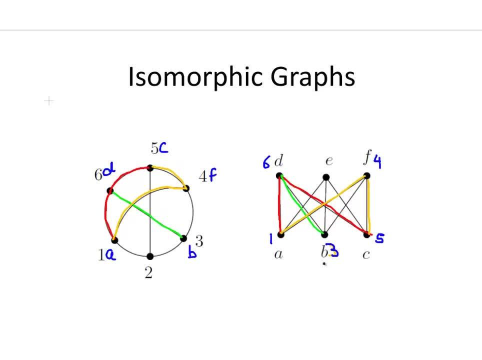 Okay, so, oh, by the way, actually sorry, we'll finish off on F. first, Magenta, down here to F, F to 3, or F to B, 4 to 3.. So far, so good. And now, finally, I want to look at these ones here- I'm going to paint them in blue- The ones that come from E to yeah, okay, that goes to A. 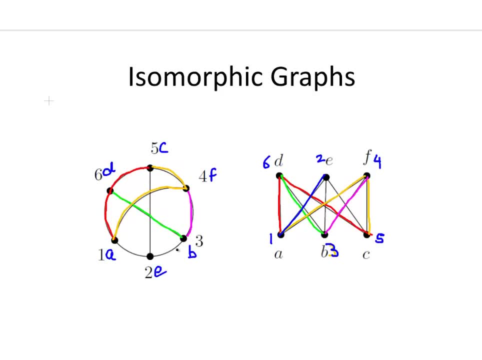 So E to A goes 1 to 2,, so it's that one there. E to B, which is 2 to 3, that one there. And finally E to C or 2 to 5, which is that one there. 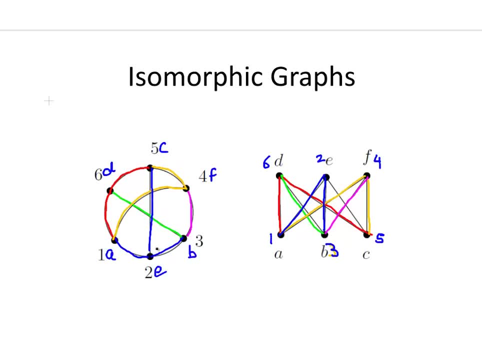 Okay now it actually would help if you had a few more colors, a very large coloring set of markers or something like that. So I'm just I'm limited to quite a few colors, but it just sort of actually would help quite a bit more. 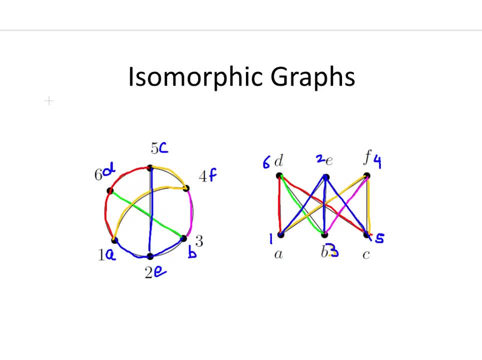 Now, that's the first one there. So we actually sort of successfully showed that the edges are equivalent to each other if we allow 6 to equal D, 5 to equal C, 4 to equal F, B to equal 3, 2 to equal E and 1 to equal A. 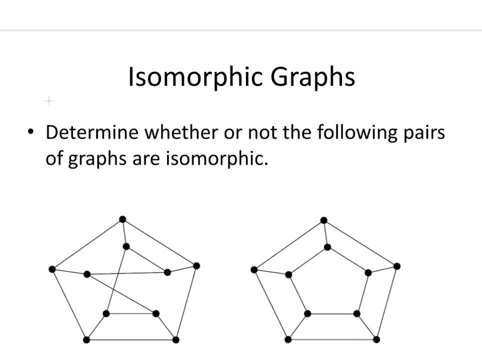 So, moving on to the next one, this one's a bit tougher. Now we have to determine whether or not these two sets of diagrams are equal to each other, So I'm just going to sort of make a bit of room there. 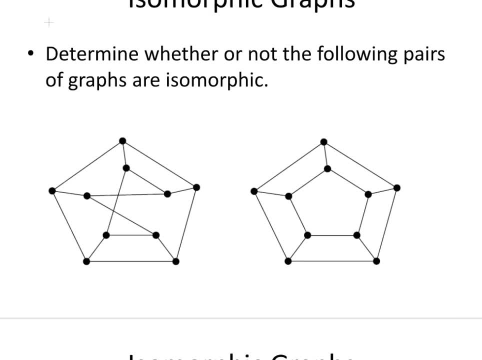 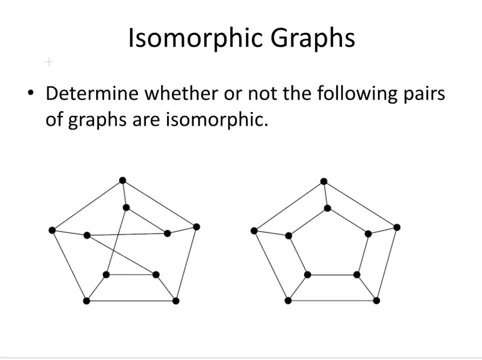 Let's go back here a second. It's like I got a bit squeezed there Now. so we have 10 vertices and they're all degree 3.. Okay, so far, so good. Yeah, we can just sort of tell that by inspection that they're all degree 3.. 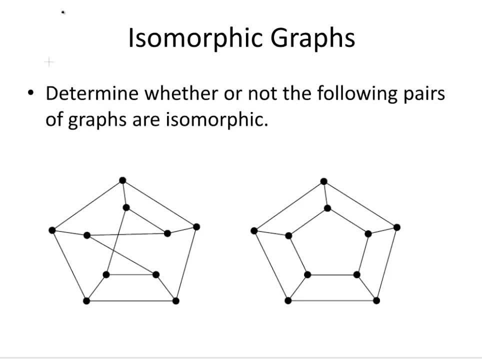 You can check it the same way as we did the last time. What is our, What is the best approach we can take here? Well, we can You try and set up the approach I've used the last time, but I'm going to just sort of propose a different approach this time. 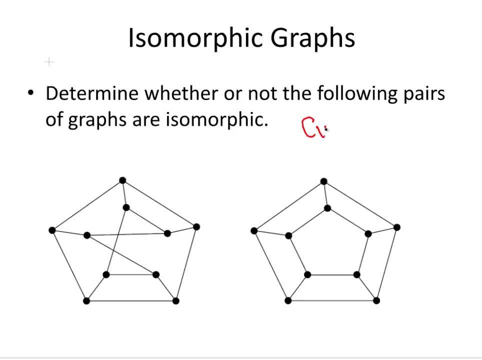 What we're going to look at is cycles this time. Okay, so this is just a sort of alternative technique to the one I've used the last time. So what we're going to do is use cycles. So here we have a 4 cycle. 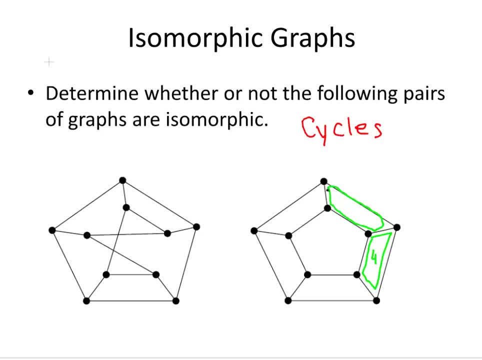 Here we have a 4 cycle. Here we have a 4 cycle. Didn't really draw that that well, This is a 4 cycle And this is a 4 cycle. Okay, and in the middle we have a 5 cycle. 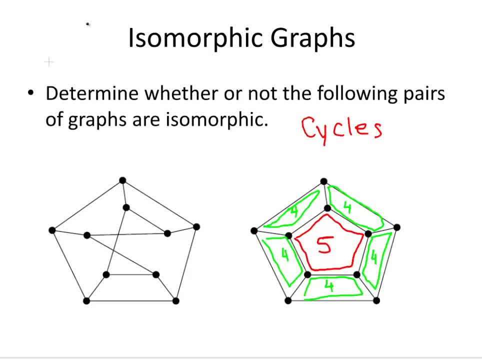 Okay, What is happening? What is happening over on this side? So we should have the same amount of 4 cycles and 5 cycles. So, first off, here's a 4 cycle. Okay, Here we have a 5 cycle. 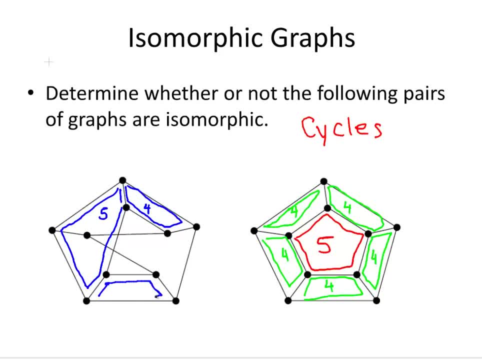 Okay, Down here at the bottom we have a 4 cycle. Okay, We automatically run into trouble here. I'm going to just paint this in. It's a different color actually. We have an extra 5 cycle here, So automatically we can tell now that these two graphs are not the same.